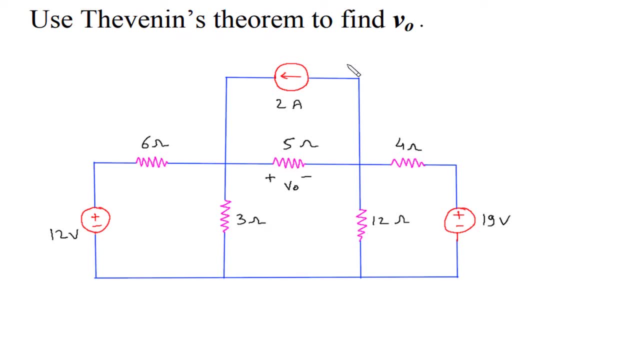 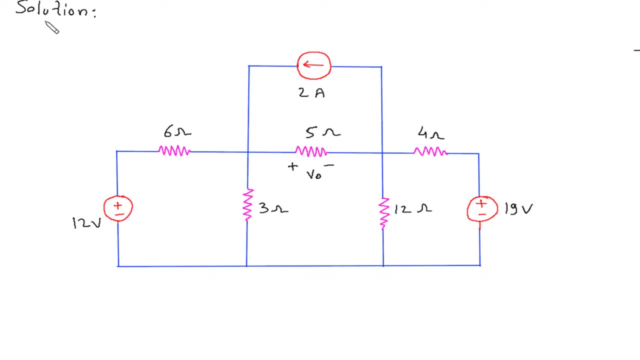 Use Thevenin's theorem to find Vo. We have to find this Vo in this circuit using Thevenin's theorem. solution: First of all, we will redraw the circuit Now. let's assume this is node V1 and this is node V2.. 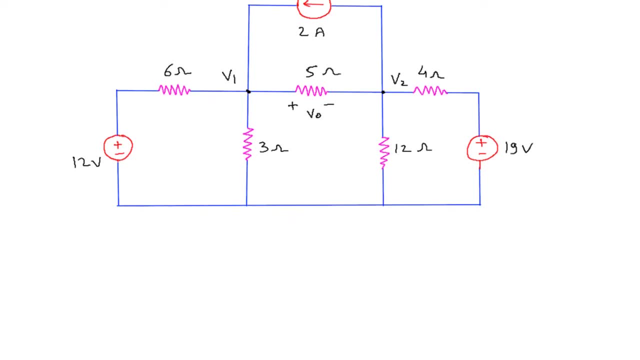 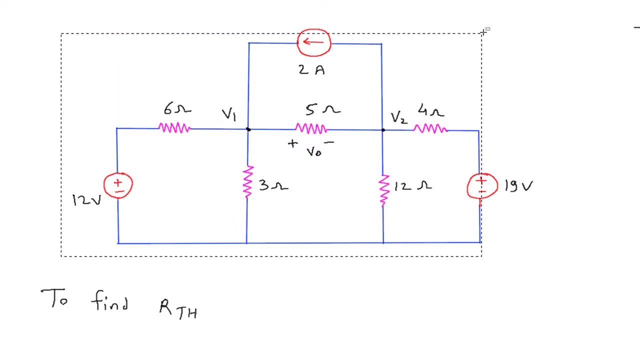 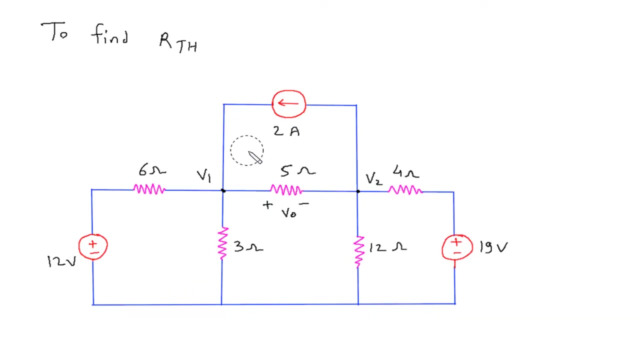 First of all we will find Rth. So to find Rth we will turn off all the independent sources. We will short circuit the voltage source and open circuit the current source. So this will be open circuited. This will be short circuited. 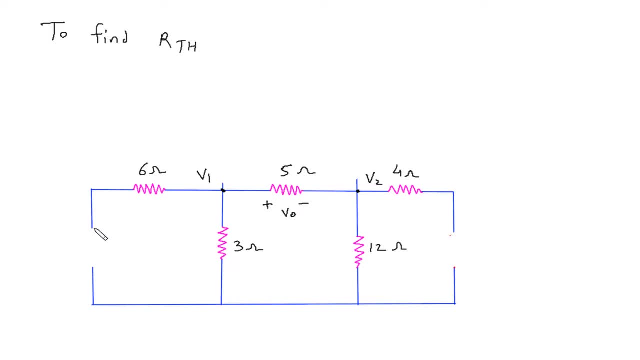 Also, this will be short circuited. This is our Rth, This is Rth, So Rth is equal to. Rth is equal to 6 Ohm parallel with 3 Ohm, 6 Ohm parallel with 3 Ohm, plus 12 Ohm parallel with 4 Ohm. 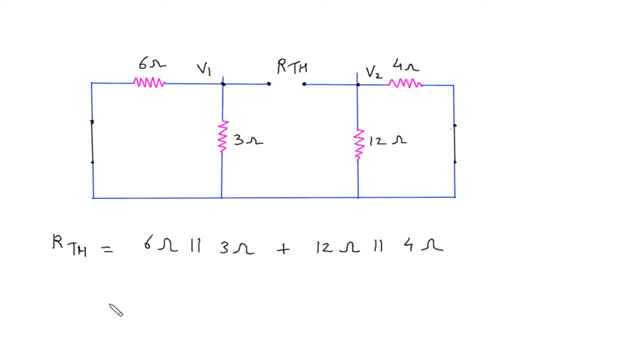 12 Ohm parallel with 4 Ohm. So this will be 6 into 3 divided by 6 plus 3 plus 12 into 4 divided by 12 plus 4.. So this will be 6 into 3 divided by 6 plus 3 plus 12 into 4 divide by 12 plus 4.. 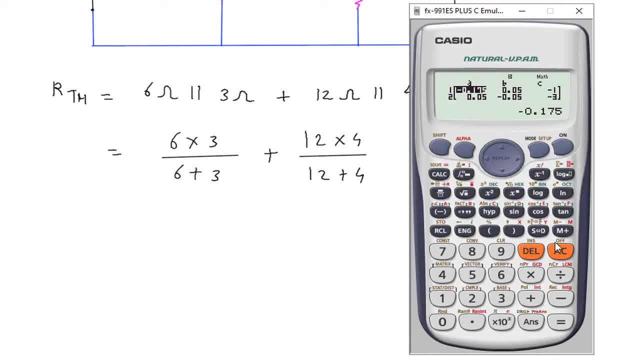 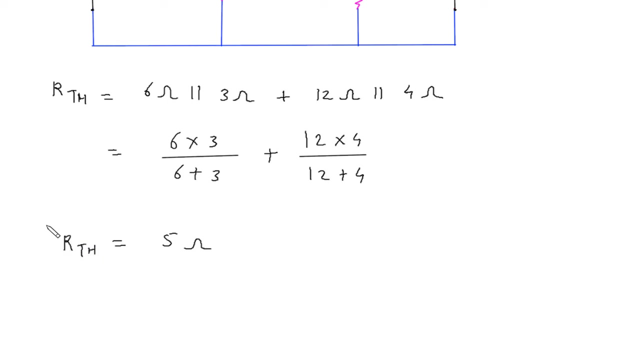 So this will be 6 into 3, divided by 6 plus 3, plus 12 into 4 divided by 12 plus 4.. 6 is 5 Ohm, so Rth is equal to 5 Ohm. Next we have to Find Vth. 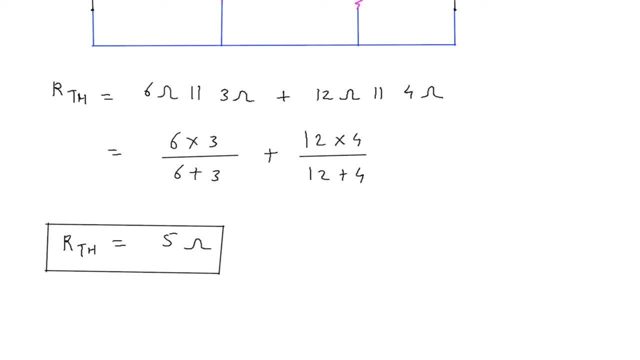 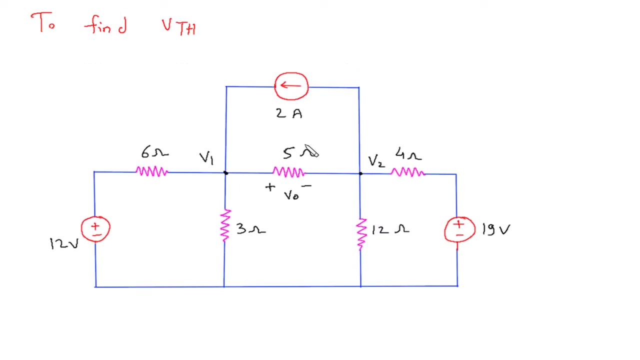 So to find Vth, to find Vth, this will be Vth, This will be Vth. We will use nodal analysis to find Vth. First we will find v1 and v2. then Vth will be equal to v1 minus v2.. 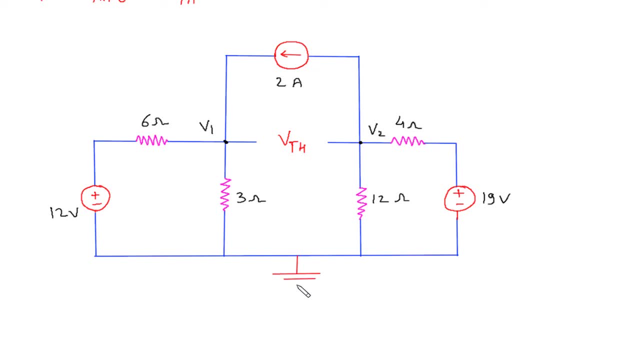 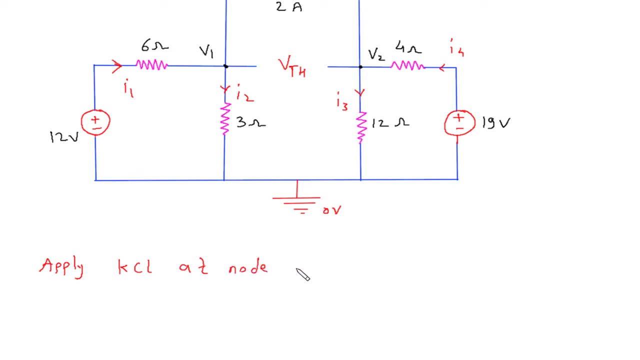 So let's assume this is reference node with zero voltage. Let's say this is current I1.. This is current I2, this is current I3 and this is current I4. So apply KCL at node V1.. Apply KCL at node V1.. 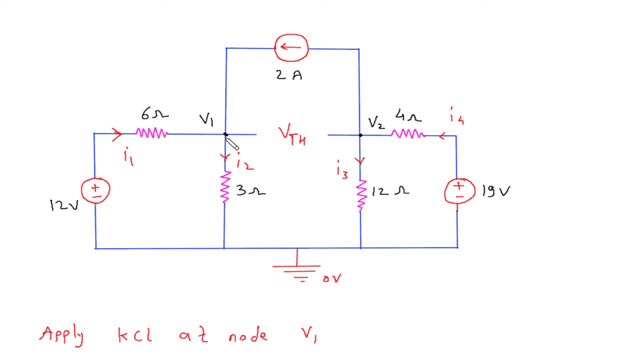 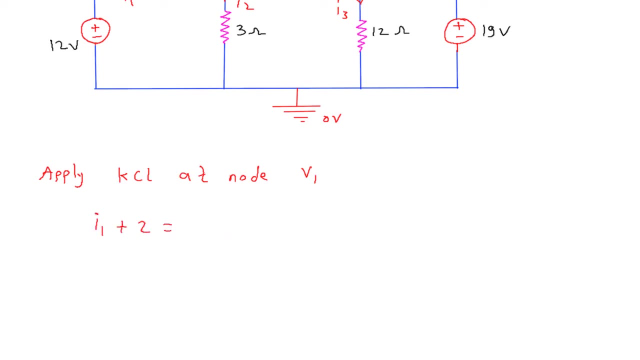 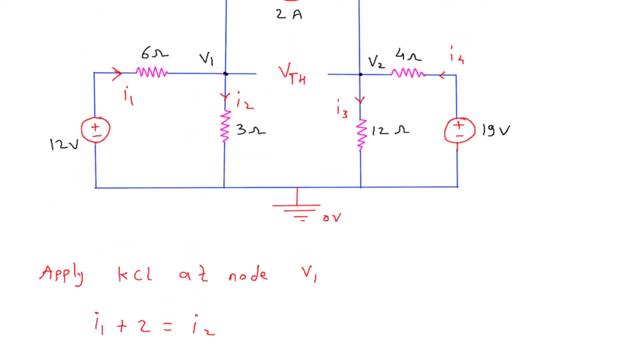 So KCL summation of all the entering current at this node is I1 plus 2.. I1 plus 2 is equal to summation of all the leaving current. Leaving current is I2.. So I2.. I1 is 12 minus V1 by 6,. 12 minus V1 by 6 plus 2 is equal to I2.. 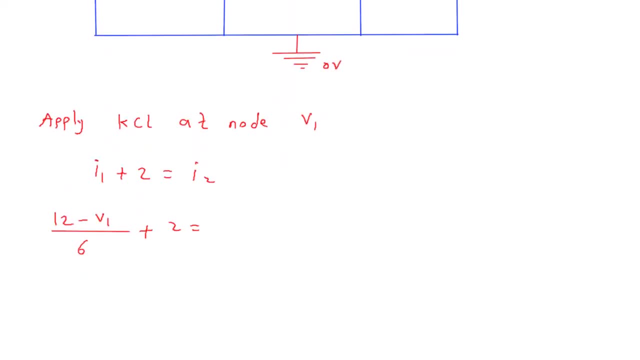 I2 is V1 minus 0 by 3, V1 minus 0 by 3.. So this will be 12 by 6 minus V1 by 6.. So this will be: 12 by 6 plus 2 is equal to or minus V1 by 3 is equal to 0.. 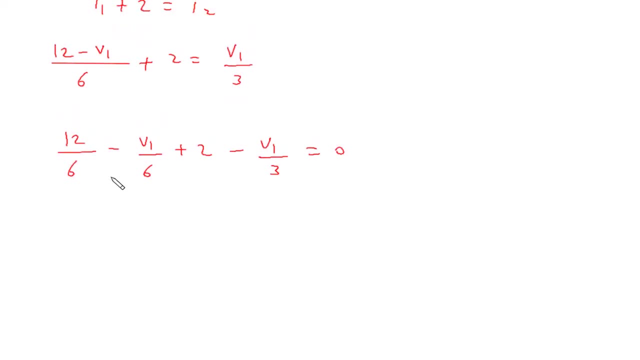 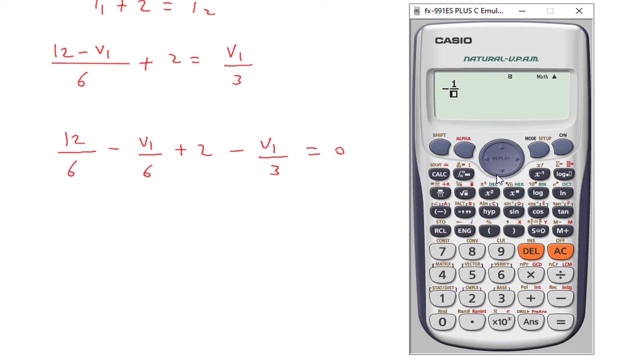 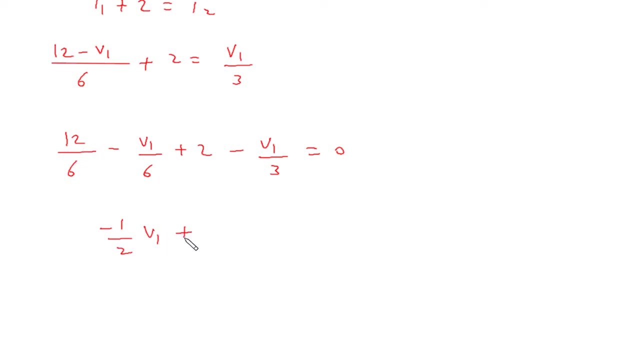 So this will be 1 by 6 minus 1 by 6 minus 1 by 3 minus 1 by 2, V1 minus 1 by 3 minus 1 by 3.. And this will be: 2 plus 2 plus 4 is equal to 0.. 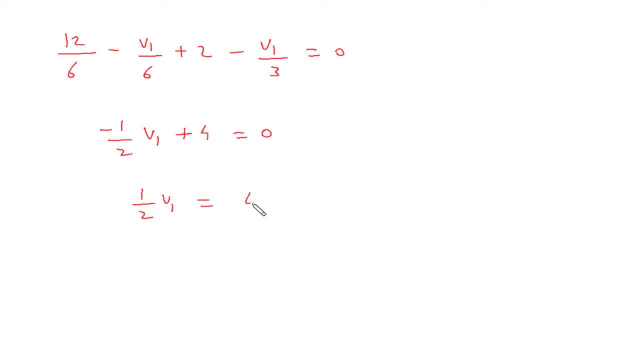 So this will be 1 by 2, V1 is equal to 4.. Therefore, V1 is equal to 8 volt. Next we have to find V2.. So to find V2, we will apply KCL. Next we have to find V2.. So to find V2, we will apply KCL. 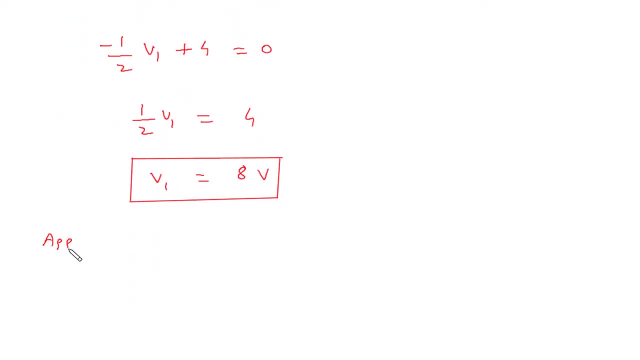 Next we have to find V2.. So to find V2, we will apply KCL. So to find V2, we will apply KCL. After this, we contracts the right. i4 is 19 minus v2 by 4.. 19 minus v2 by 4 is equal to i3.. i3 is v2 minus 0 by 12.. v2 minus. 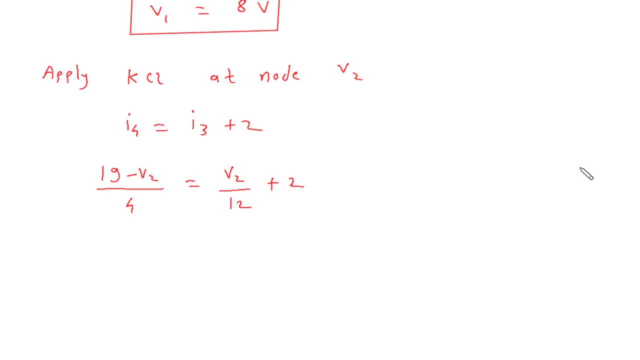 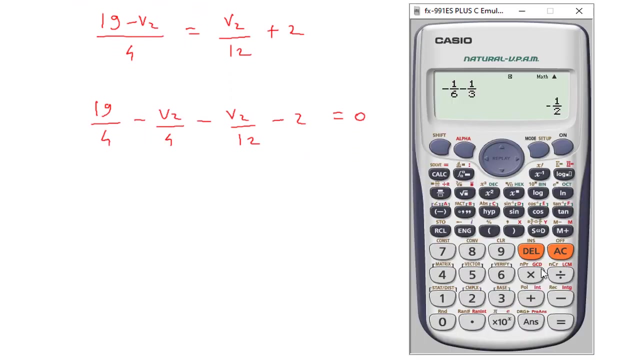 0 by 12 plus 2.. So this will be 19 by 4 minus v2 by 4 minus v2 by 12 minus 2 is equal to 0.. So this will be minus 1 by 4, minus 1 by 12. 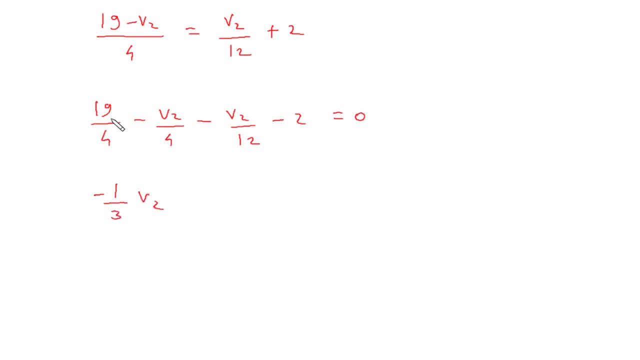 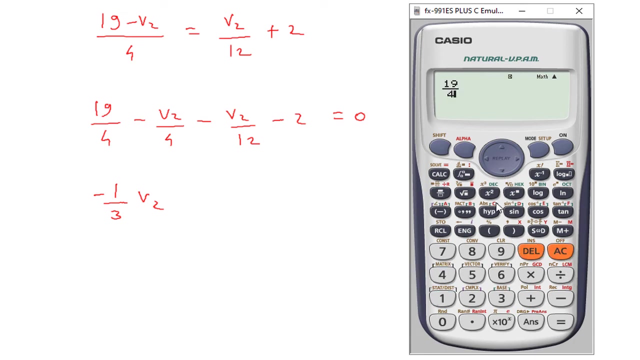 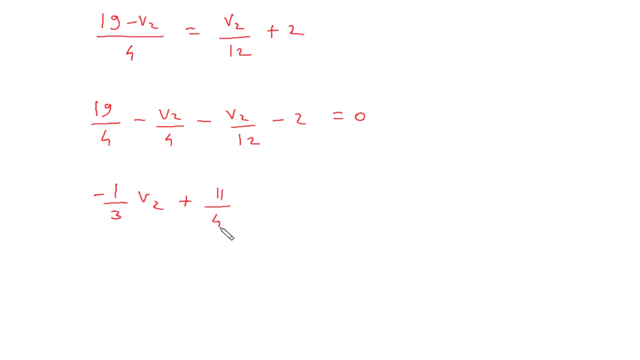 minus 1 by 13 minus 1 by 14 minus 1 by 15 minus 1 by 16 minus 1 by 17 minus 1 by 18 minus 3. v2, this will be 19 by 4.. 19 by 4 minus 2. 11 by 4 plus 11 by 4 is equal to 0. So. 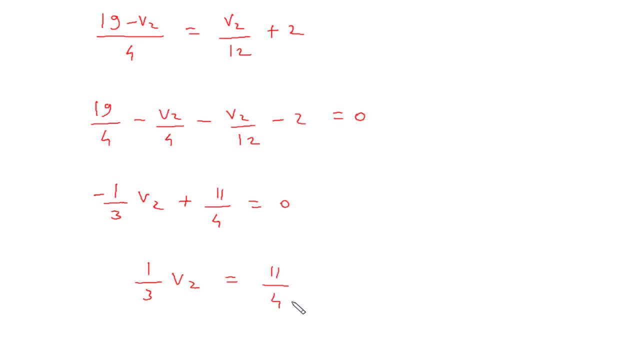 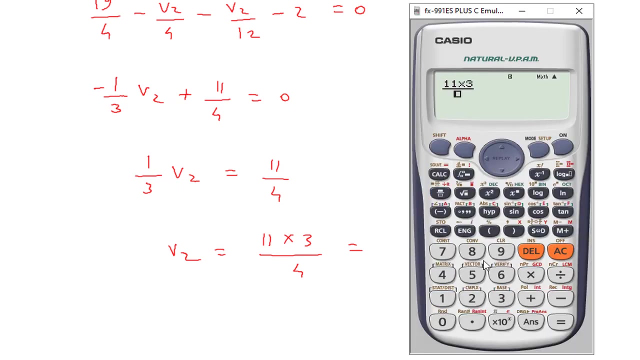 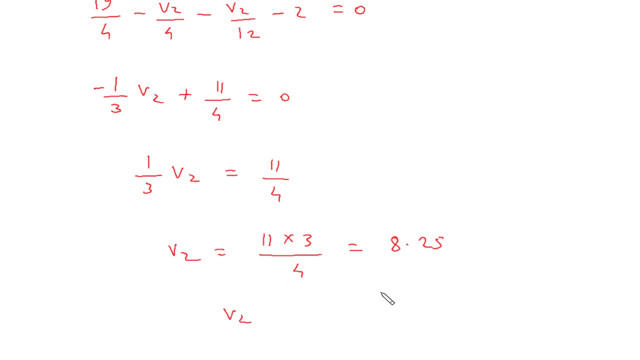 this will be 1 by 3.. v2 is equal to 11 by 4.. From this, v2 is equal to 11.. 11 into 3.. By 4. 11 into 3 by 4 will be 8.25.. 8.25.. This is the value of v2.. 8.25 volt. We have to. 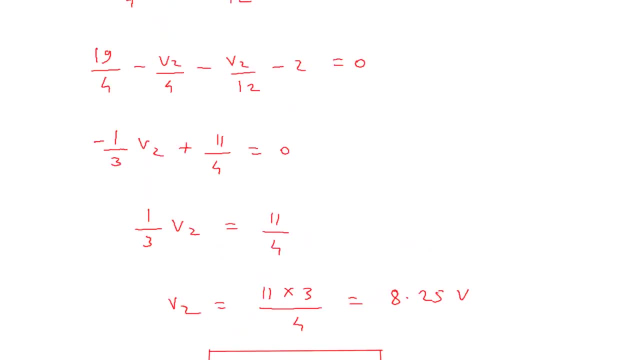 find vth. vth is equal to v1 minus v2.. v1 is 8 volt And v2 is 8.25 volt, So this will be 0.25 volt. vth is equal to minus 0 point minus 0.25 volt. 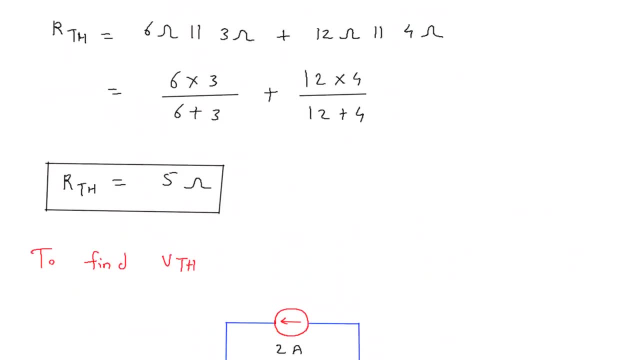 Now from this we can draw the evening equivalent circuit. This is rth And this will be vth. The direction of vth will be like this: This will be positive And this will be negative Because it is minus 0.25.. 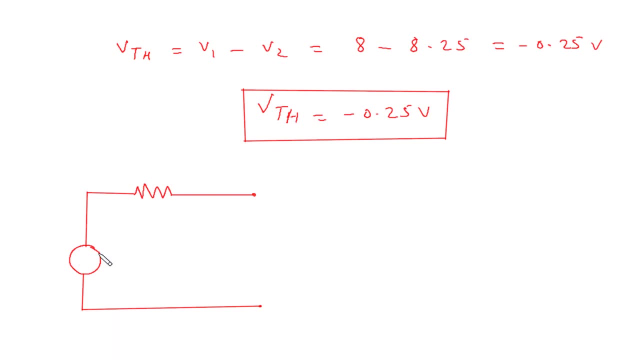 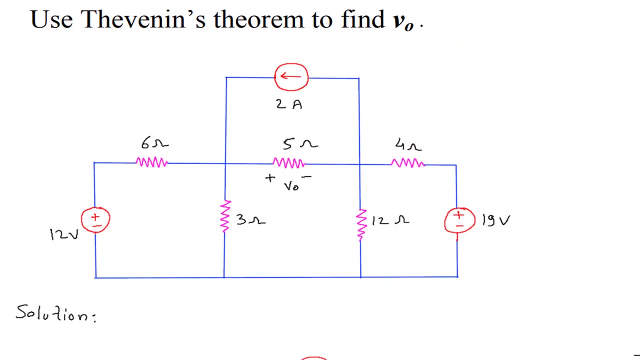 Or we will draw like this default Thevenin theorem: this will be positive and this will be negative, and this will be minus 0.25 volt, and this is Rth, this is Rth and this is Vth. Rth is 5 Ohm, this is 5 Ohm and this is RL. or we have to find Vo using Thevenin's theorem. 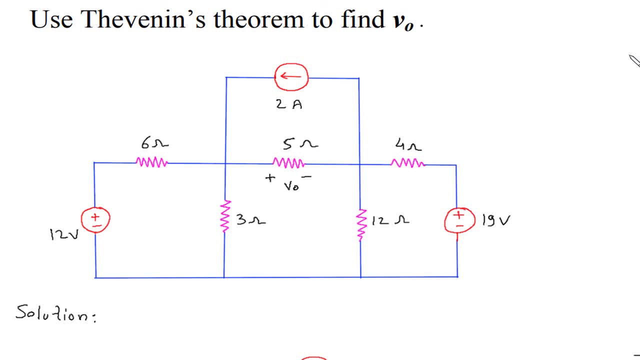 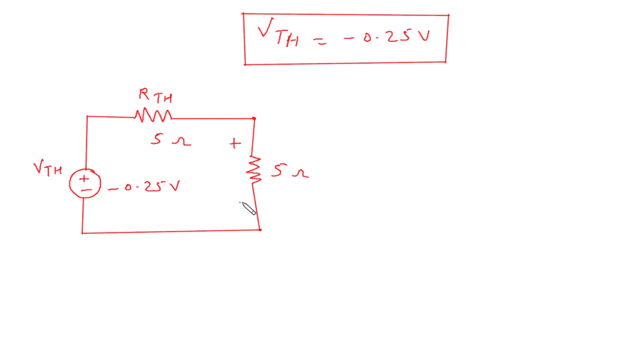 so this is 5 Ohm plus minus Vo. This is 5 Ohm, This will be plus, this will be minus, this is Vo. So we can apply voltage division rule here. apply voltage division rule, So this will be: Vo is equal to this voltage, which is minus 0.25, into this resistance, which.